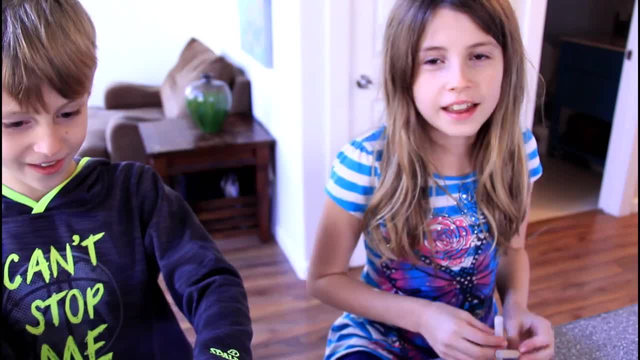 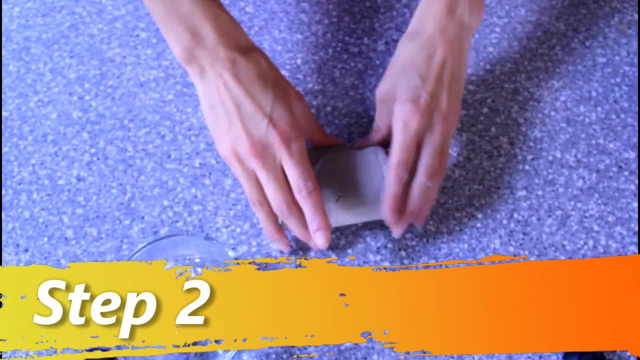 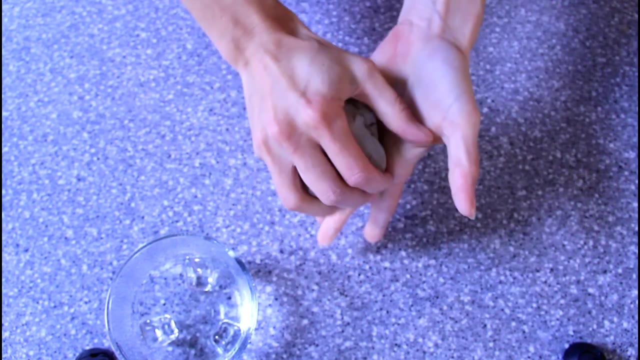 And that's considered pottery. I'm going to create a flower pot. I'm going to create a teacup, Okay, So grab yourself some water and a big slab of clay. What you want to do is you want to warm up your clay by smooshing it in your hand. 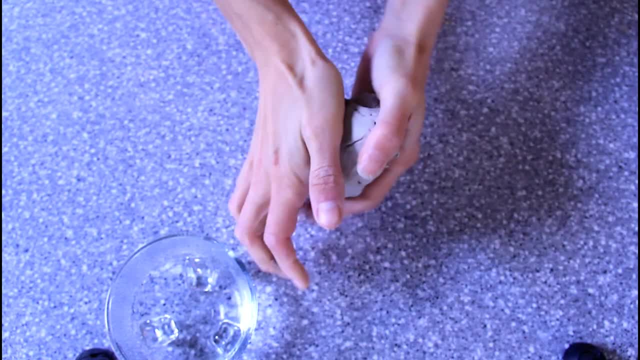 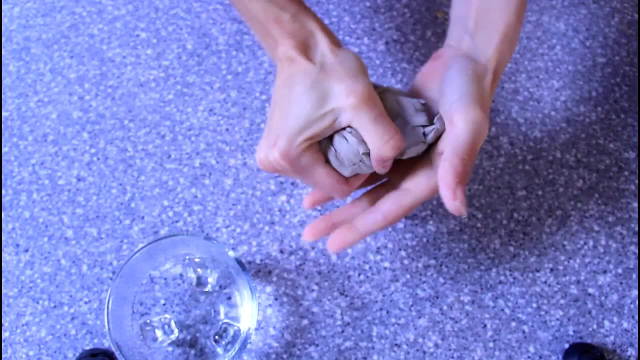 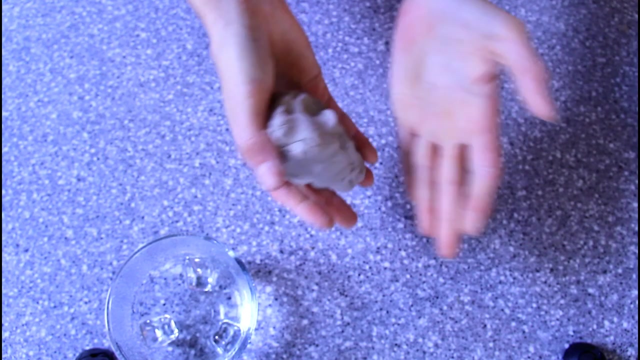 Smoosh it for a little while until you feel it getting a little bit more warm, And then you can start forming it into a ball. Okay, This will make it easier to work with. So now you can either try to form in a ball with your hands, like this: 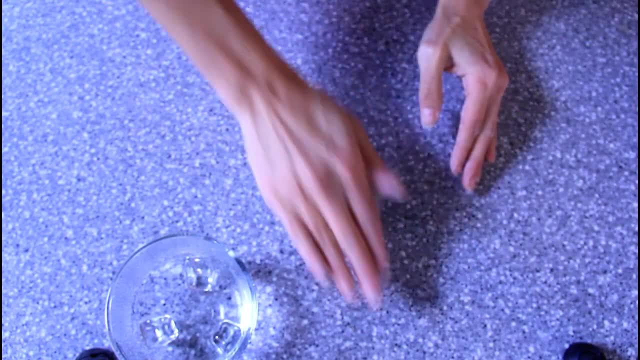 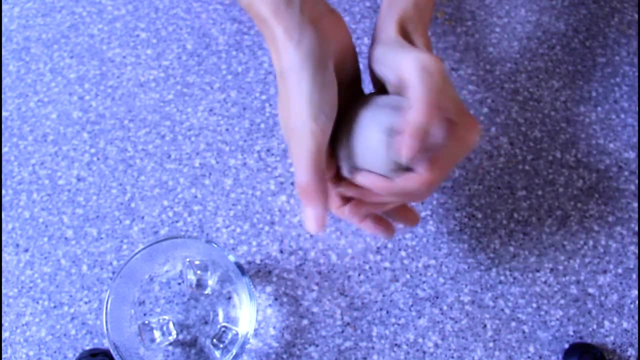 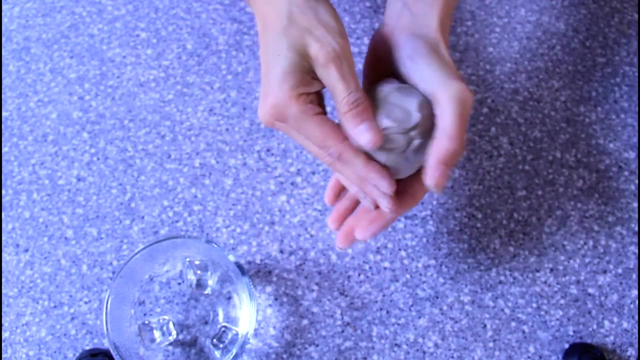 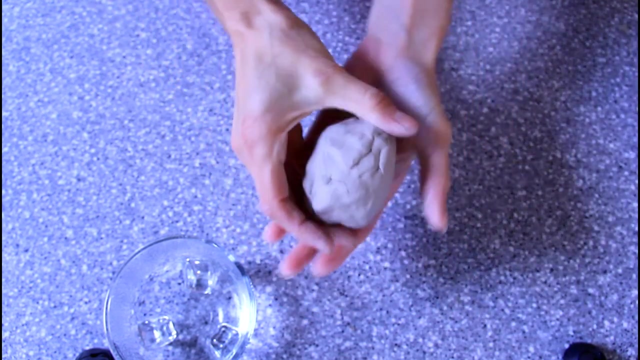 Or you can use your table and roll in the ball like this. So whichever one works better for you, Go ahead and try both. Okay, Now, the circle does not need to be perfect, But notice how there's cracks like that. You don't want to have any cracks like that. 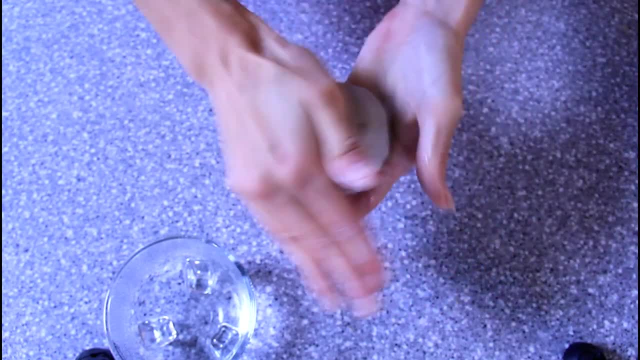 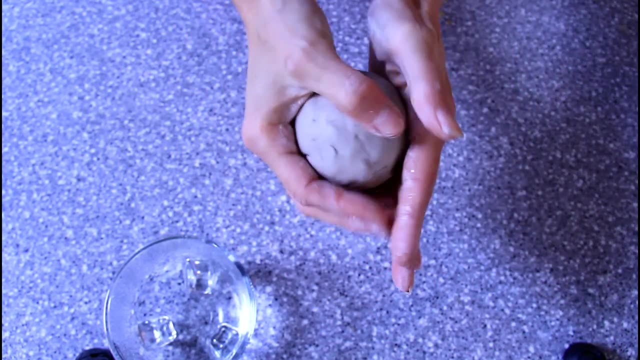 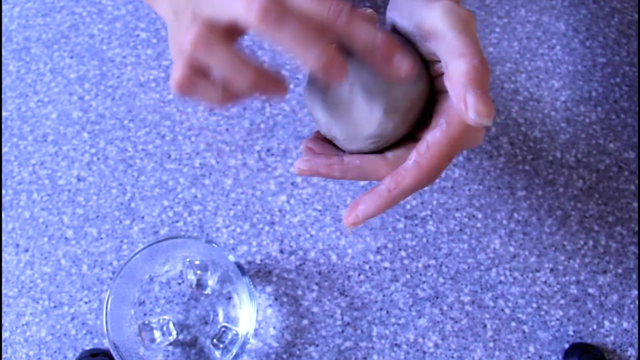 Because when you start to form your pot, Whatever pot you're using, Whatever you're making, The cracks will get worse and worse, And then you'll have cracks inside of your pot And that's not good. So see how I'm just taking my finger and going over those cracks. 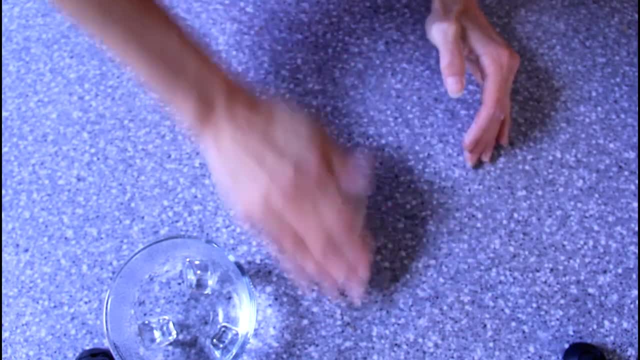 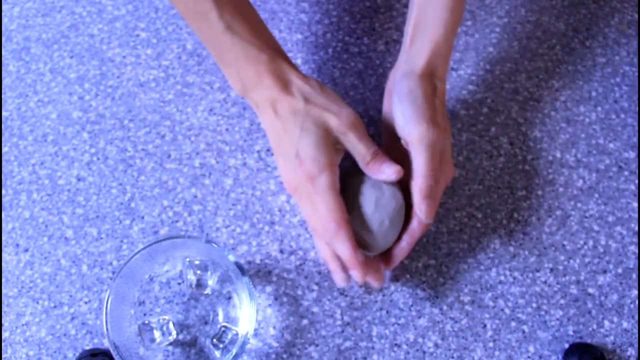 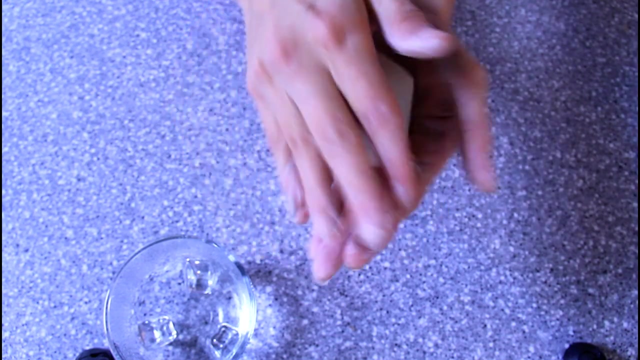 And I make sure and roll it to fill in those cracks So they don't make little bubbles. See how nice and smooth that is. Let's do it to the other end. Okay, See how it's kind of like a cone now. 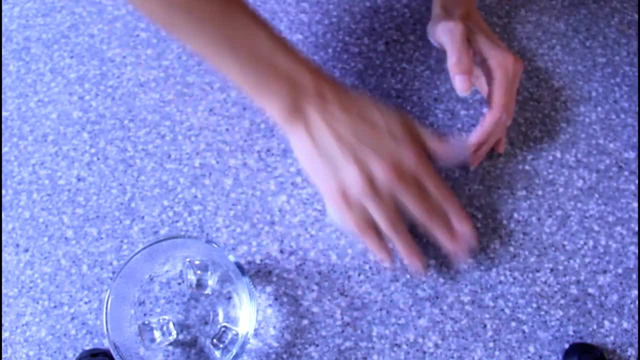 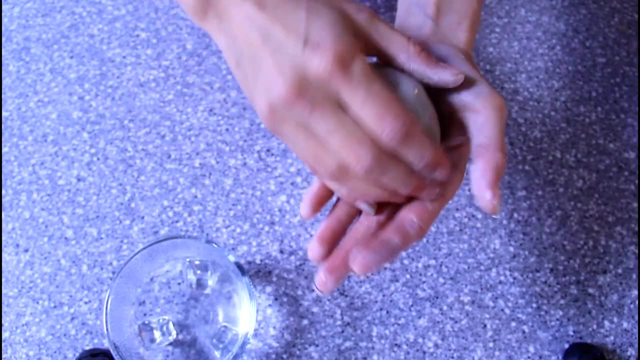 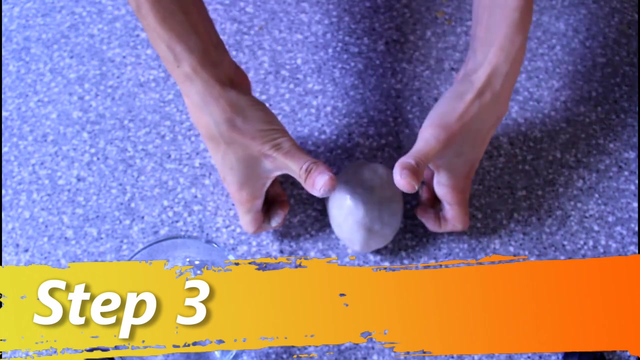 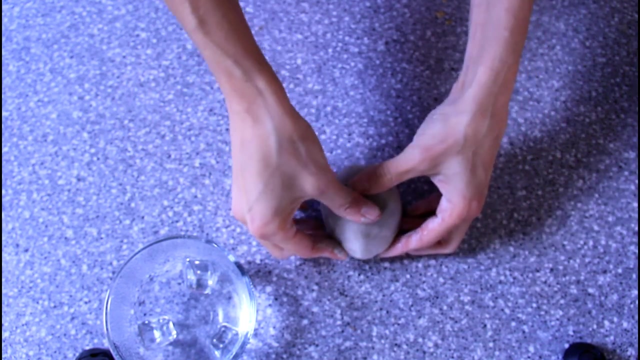 Just keep rolling that, So I'm going to put a nice layer of water over it, Not too much. Now what I can do is push with my thumbs down into the middle. Now, this is exactly what you need to do to make a pot. 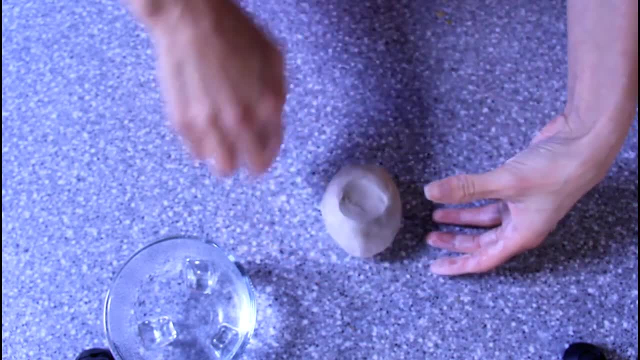 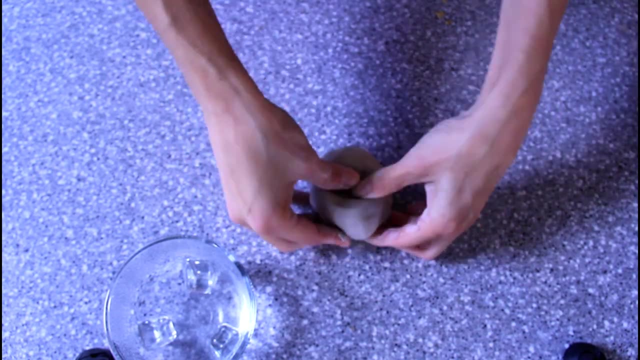 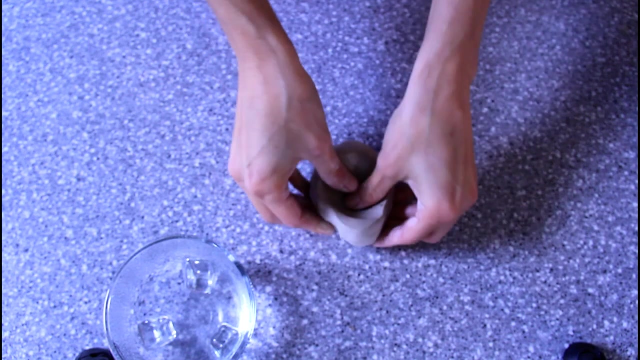 When you're on a pottery wheel. Okay, I'm assuming you guys don't have a pottery wheel, But if you do, You can do the same thing on your pottery wheel. It'll just form a lot faster. So see how I'm forming the pot shape with my hands. 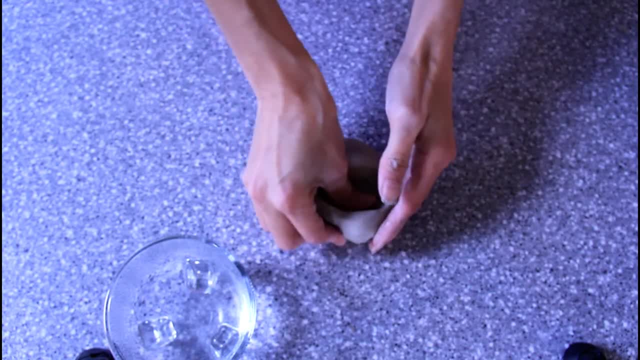 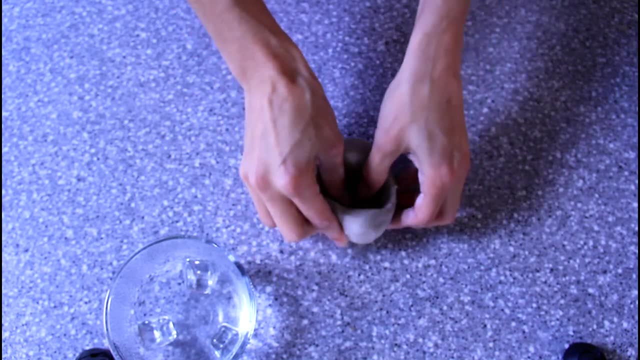 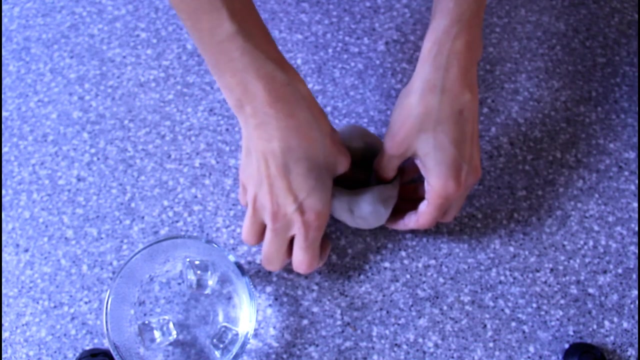 And my thumbs are pushing in. Now you want to make sure that when you're pushing in With your thumbs, That you know the distance on the bottom from your table So you don't create a hole in the bottom, So you don't want to go too far. 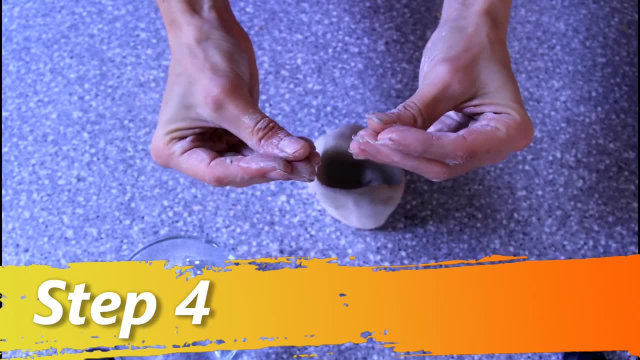 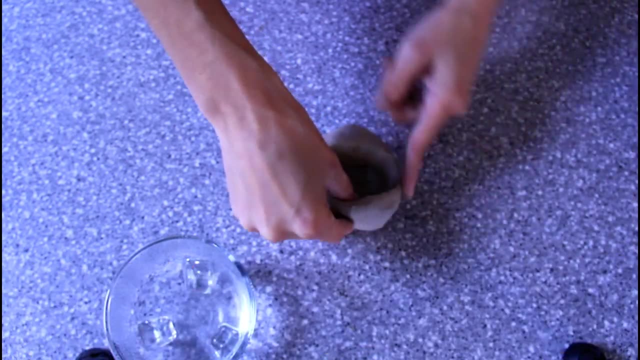 Now the next step is you're going to pinch Again. if you're on a pottery wheel, You would pinch, And where you're pinching, This whole thing would become the size of your pinch. So you just go around in a circle like this. 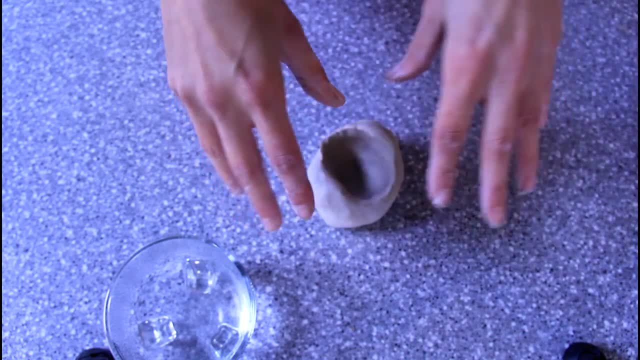 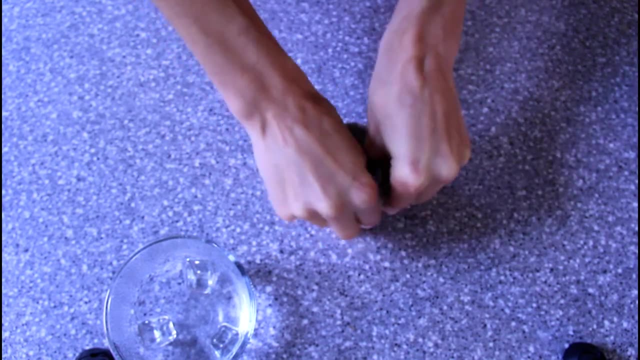 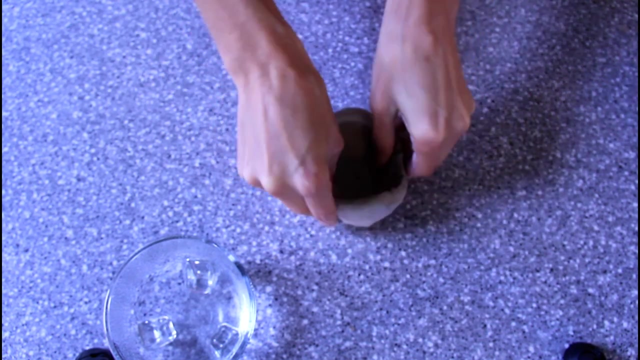 Okay, But since we don't have a pottery wheel, We can still do our best And we just pinch around it Like this Kind of rotating it around. Okay, Some sides will be thicker than others, But don't you worry. 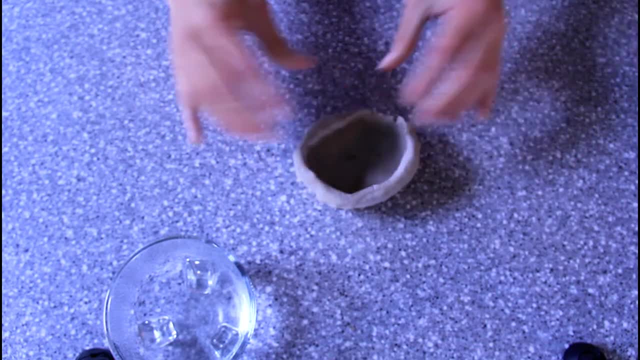 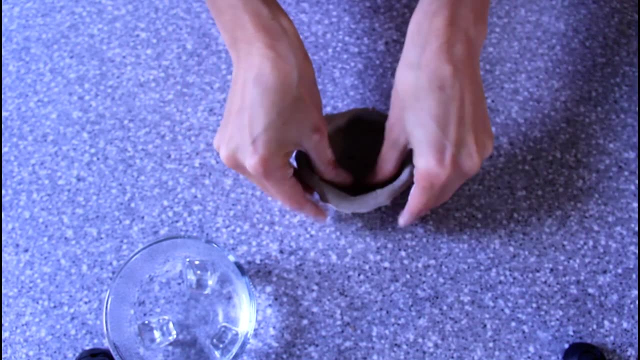 We will take care of that when we get to the end. Now it depends on what pot you want to make, But this pinching technique will get you to the pot you want to make. So, for example, Look at this teacup. 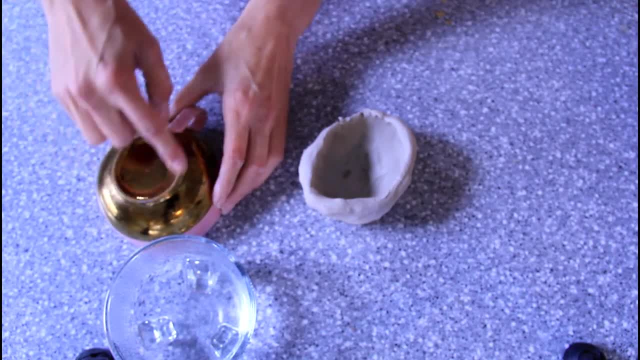 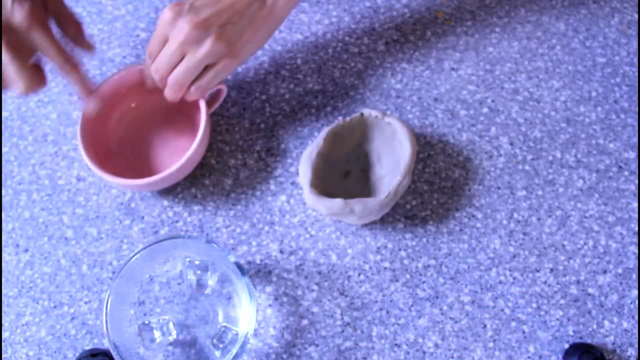 Okay, The bottom of the teacup has a circle, And then it gets round As it goes up, And then it's pretty flat, Okay, So what I want to do If I'm going to make a teacup: 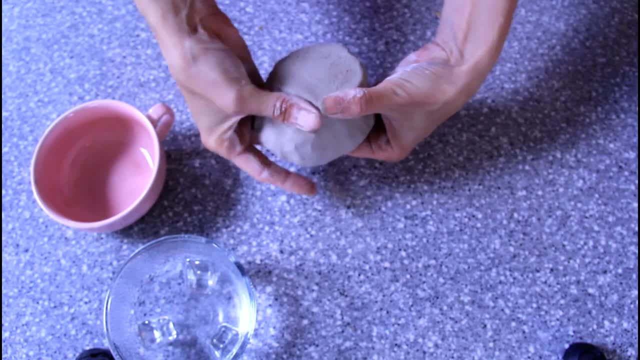 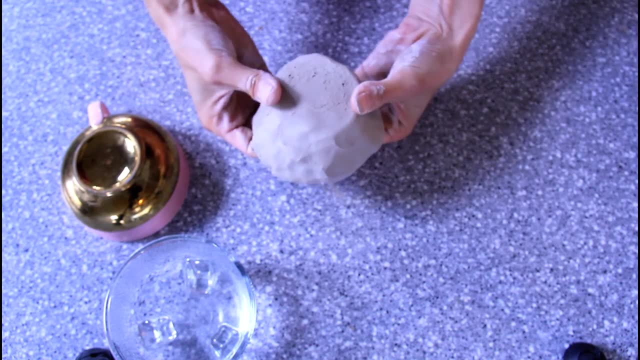 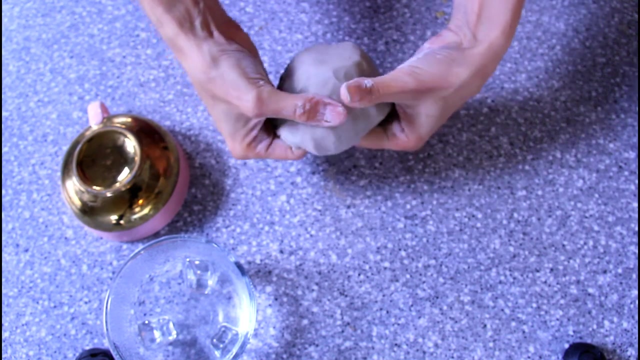 But you can make whatever you want Is: I want to make sure that I have The small circle on the bottom, So I'm going to push Until I get about the size of that small circle. Okay, You see this right here. 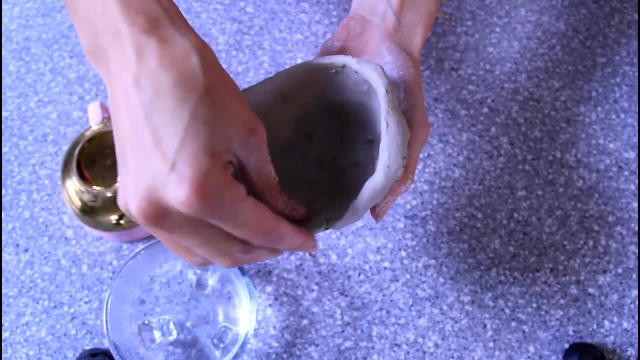 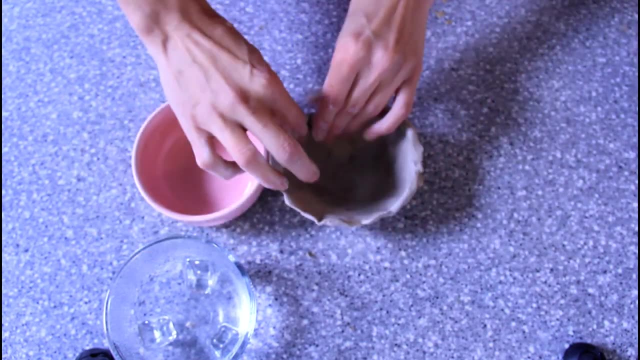 This is because it's starting to dry out, So I'm going to take some water And put it right over there. See, Am I getting as high as the teacup? It's getting closer, So I notice that it's really thin over here. 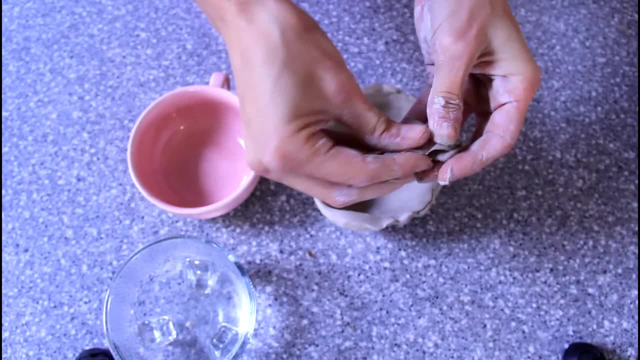 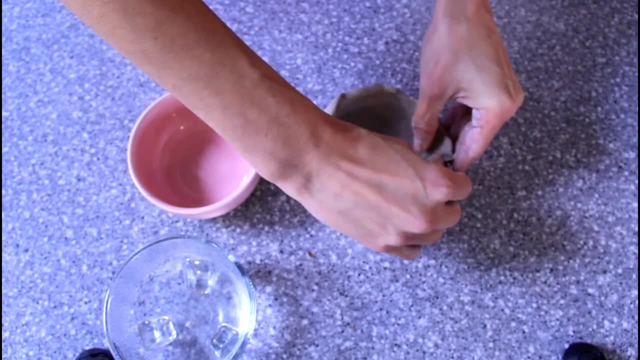 So what I'm doing Is I'm grabbing some clay And I'm flattening it out With my fingers And then I add it to that side And then I smooth it in. What it looks like Doesn't matter so much. 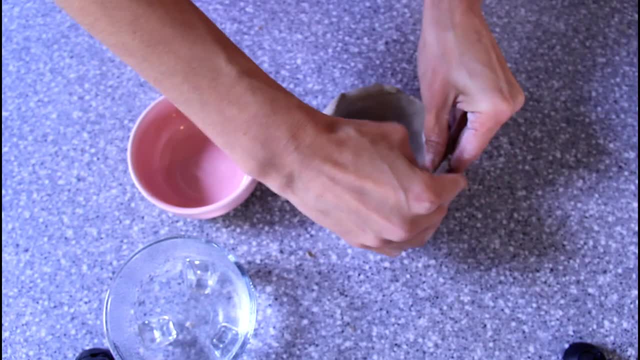 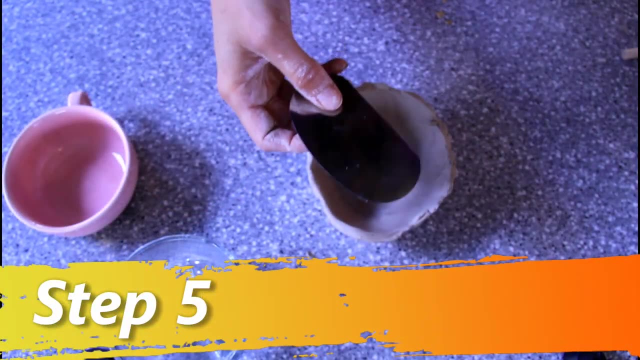 As what we're learning, As we're creating, Okay, And I make sure that there's no cracks. So what I'm going to do now Is I'm going to grab some tools. I'm going to grab my kidney tool here. 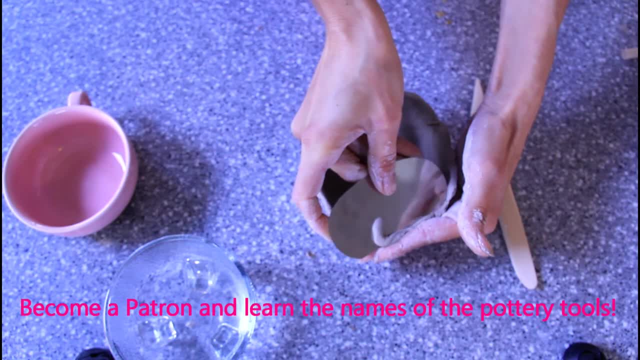 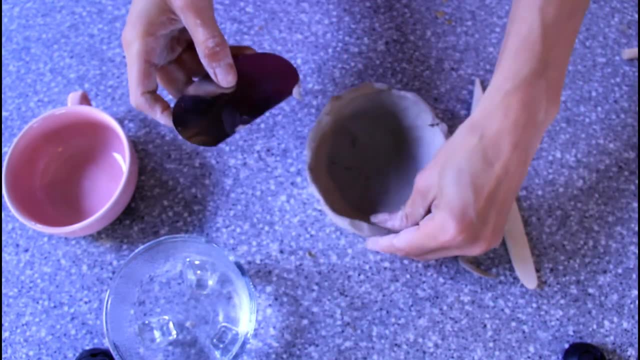 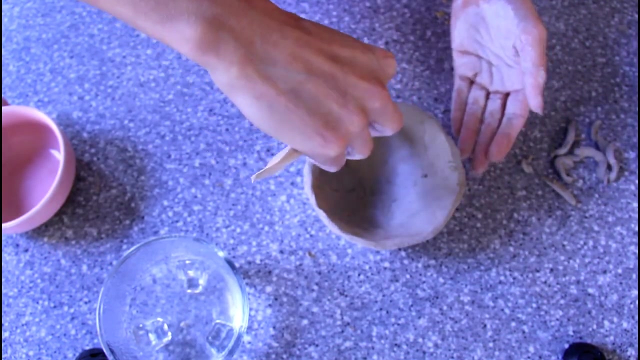 And I can cut away The top, Pushing against it, So that top of it Is all the same size. So I just go around. So now I'm using this tool To smooth out the top. Alright, So that's going to be nice. 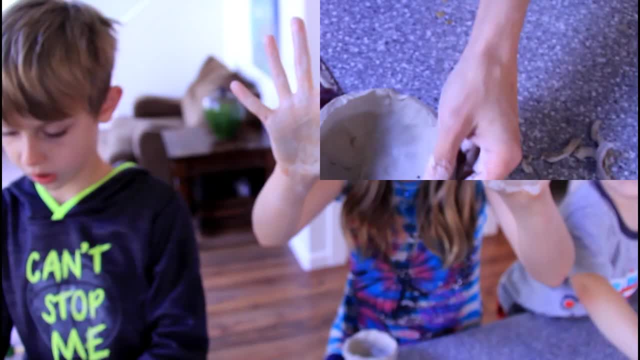 Like this. I'm just using this as a guide. I'm making a flower pot. I'm making a flower pot. You can't be saying that. Well, you already made a little tiny teacup, So You want to make a flower pot too? 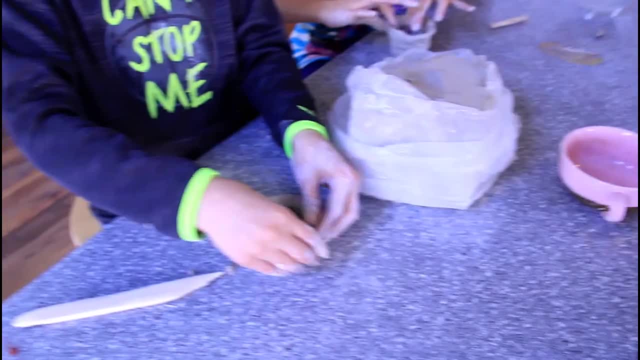 You can make as many projects as you want. Okay, Yay, I'm a pottery. Thank you for creating with us. Let us know in the comments if you have any questions And we'll see you next time. Bye, Bye. 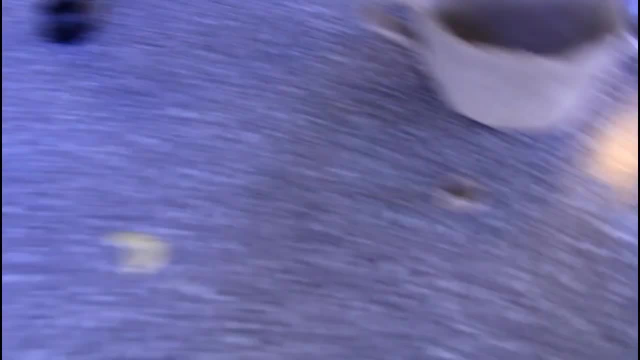 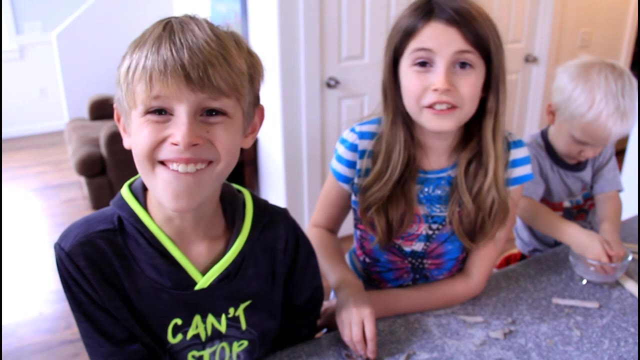 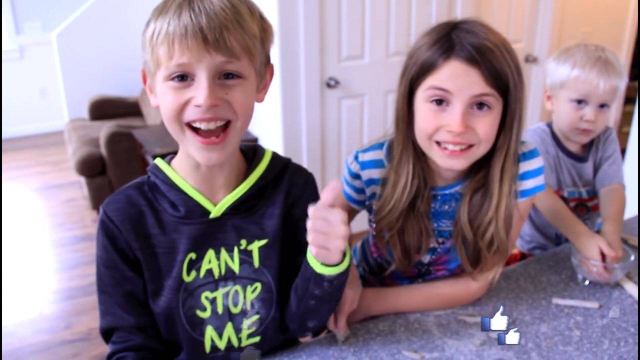 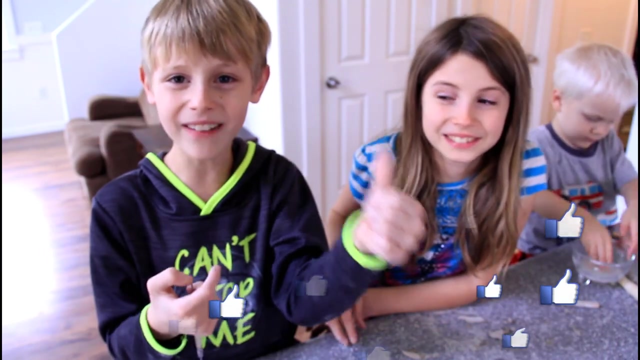